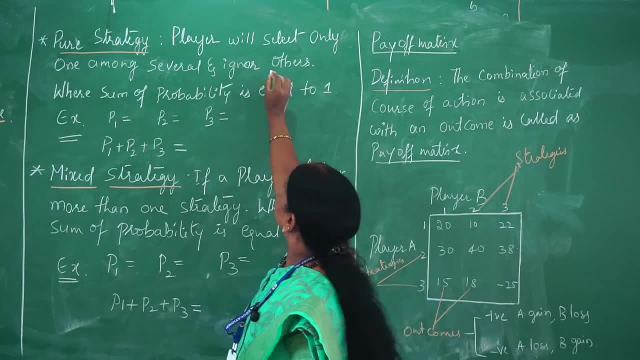 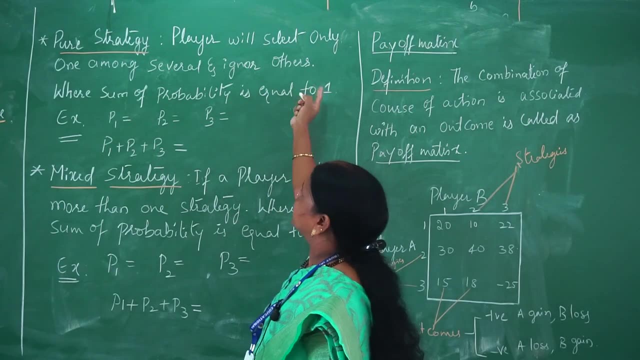 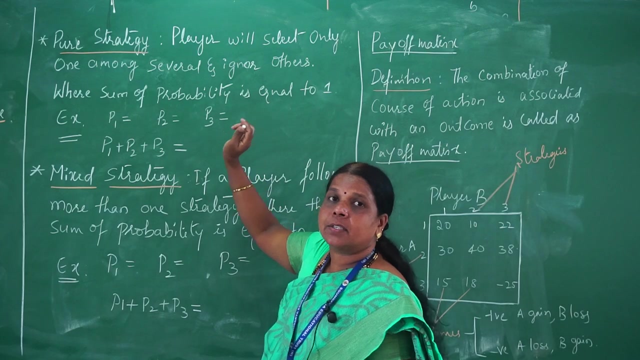 mixed strategy. The pure strategy is like this: A player will select only one among a several strategy that is called as in pure strategy, and other strategies can be ignored. There may be several strategies for the player, but he won't select all the strategy. He will select only one. 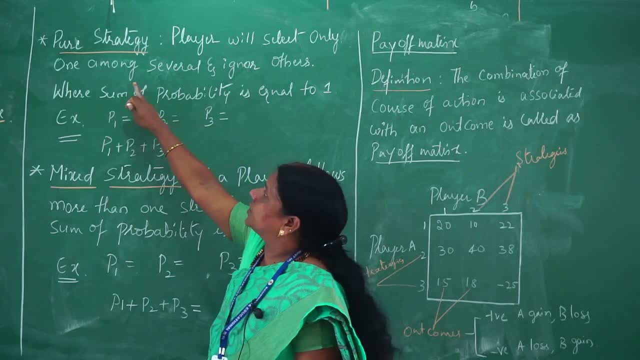 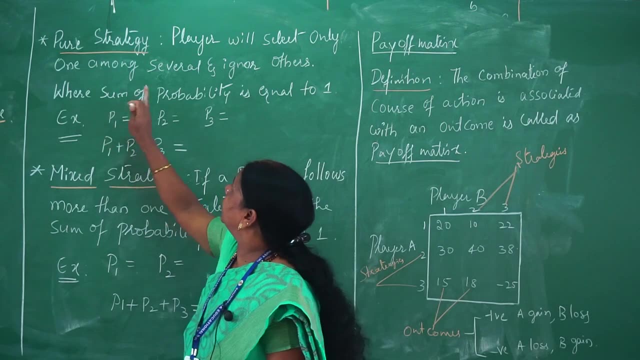 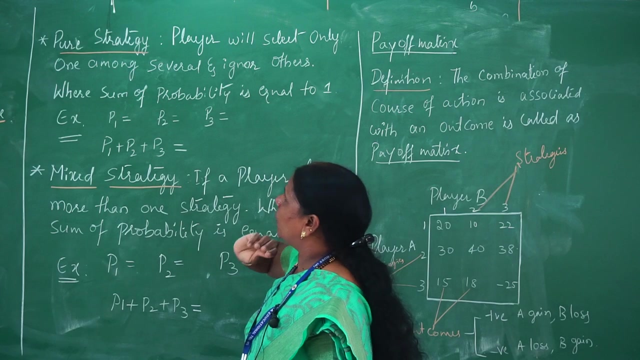 strategy among the several. So such kind of an strategy is called as in pure strategy, And here the strategy whichever he is selecting player that should be there. we are finding the probability like this, where sum of all the probability is should be equal to one. 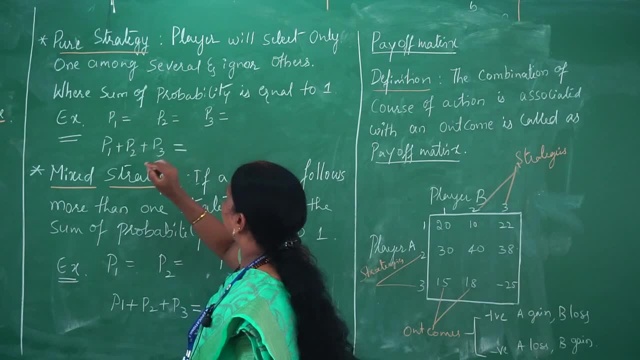 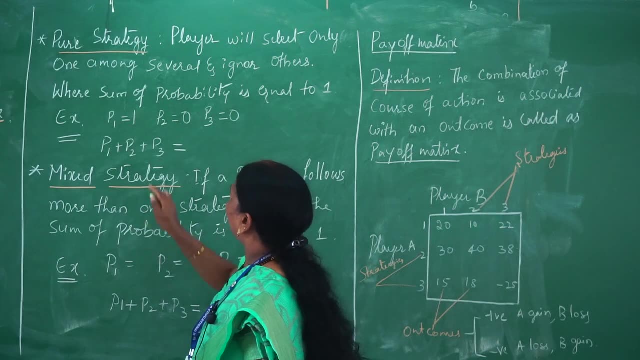 For example, there are three probabilities: P1, P2, P3.. If he is choosing only one strategy, P1, then P2 and P3 should be equal to zero and the sum of all these should be always equals to zero. This is the condition for evaluation. 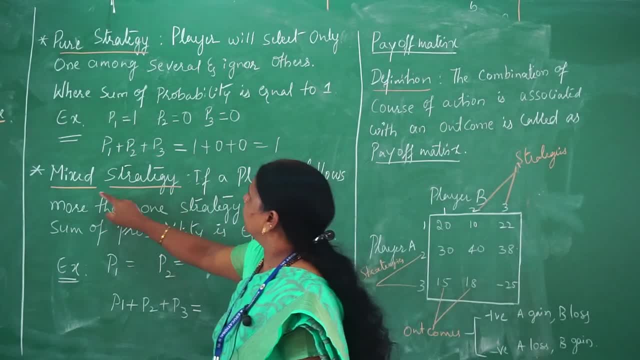 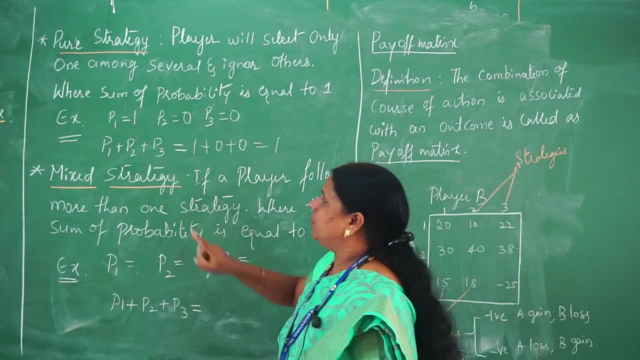 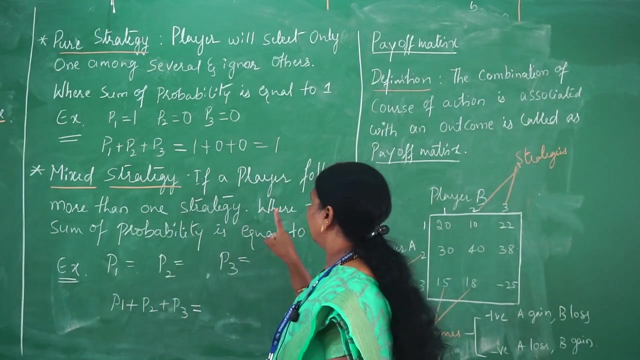 Okay, So this is the condition for evaluating the probability. Moving to the next mixed strategy, If a player follows more than one strategy, then it is called as a mixed strategy. Again, here we need to find out the probability, where the probability of sum of each and every should be: each and every probability should be equal. 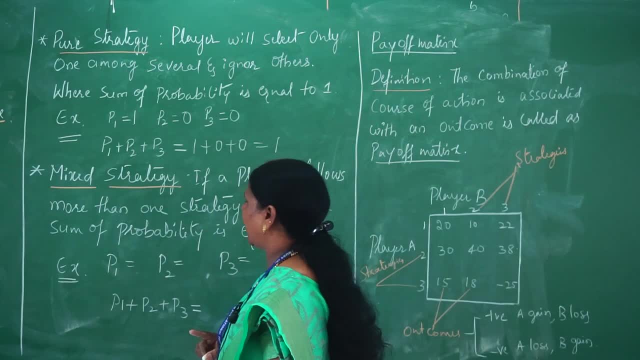 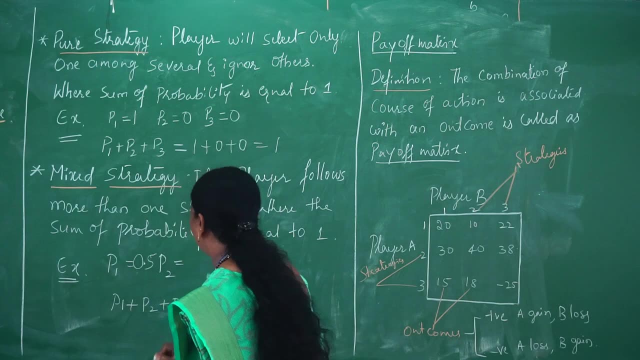 to one. So if he is selecting more than one probability or strategy for that, we need to find out here the probability like this: P1 equals zero, P2 equals to 0.5, but P3 equals to 0. after evaluation of this addition, of all these probability, 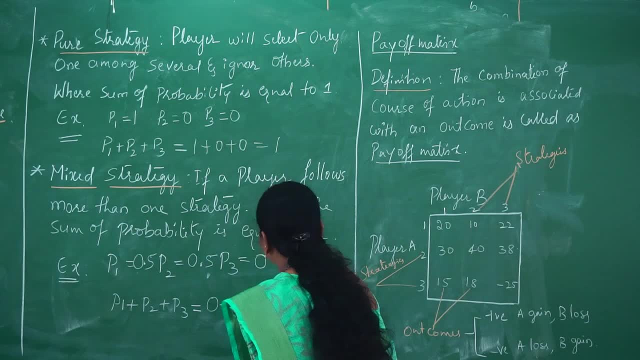 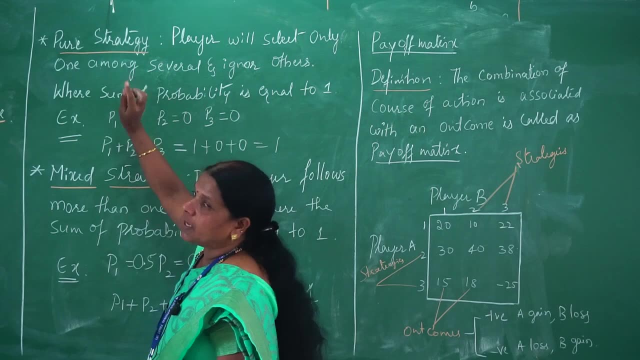 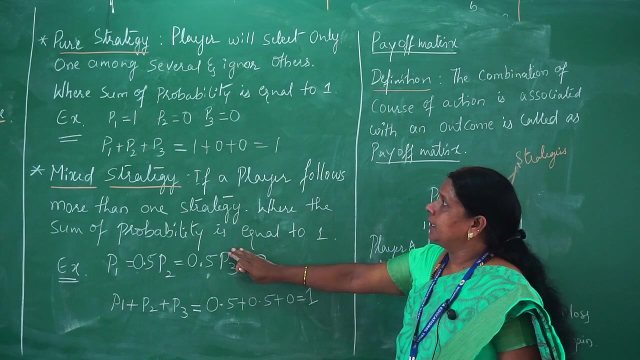 0.5 plus 0.5 plus 0, it is always equals to 1.. This is the condition for evaluating mixed strategy probability as well as the pure strategy probability. So, moving to the next, if you wanted to apply the probability of mixed as well as the pure, 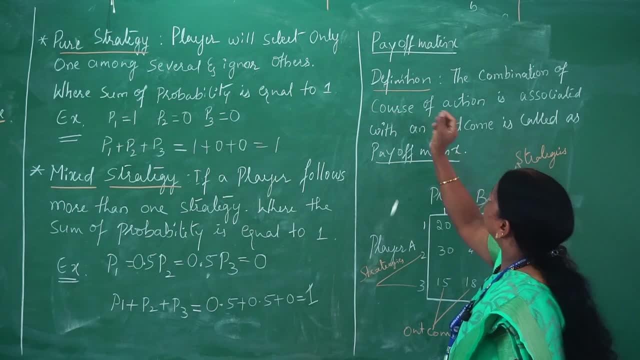 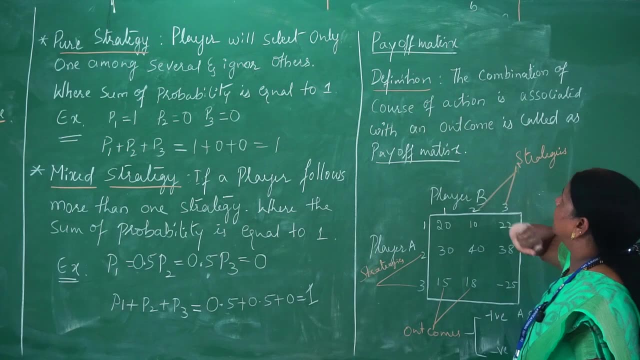 strategy probability. So if we want to apply the probability of mixed strategy towards one of the concept called as a payoff matrix, then we need to define the definition. The definition of payoff matrix will be defined like this: The combination of courses of action. that is nothing but course of action, just know. 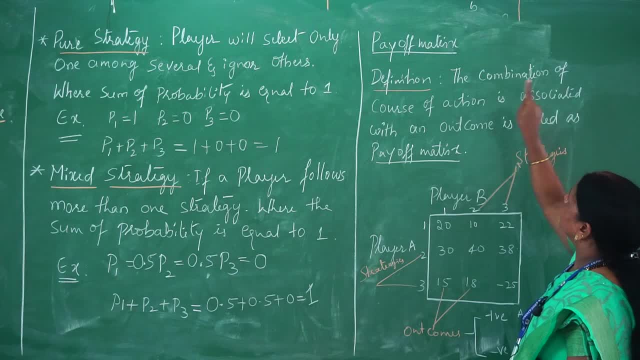 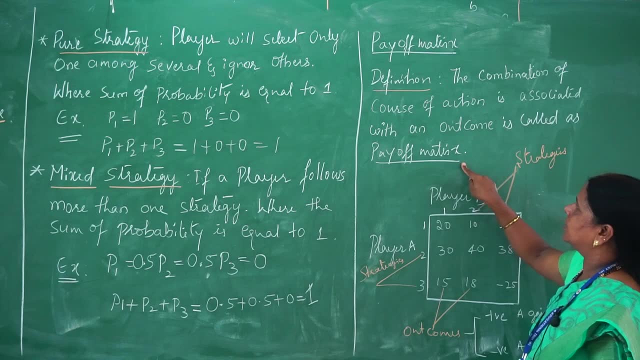 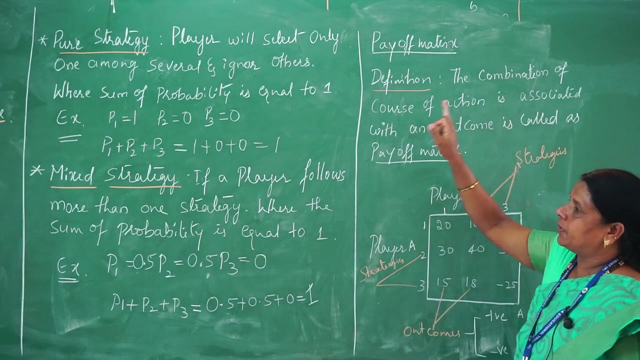 we discussed, it is called as a strategy. The combination of strategy is associated with an outcome, is called as an payoff matrix. So, whichever the matrix we are defining, They We need to define a outcome. that outcome is associated with the strategy, So that strategy itself is called as a course of action. 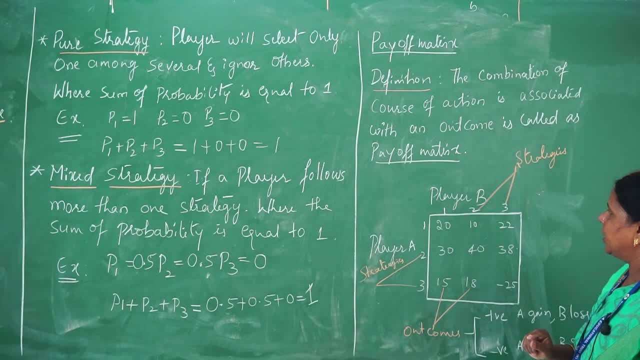 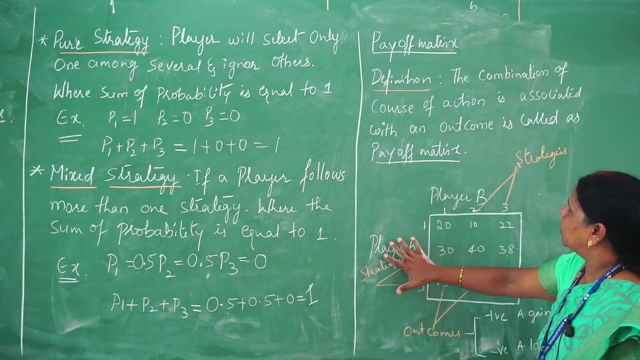 Here is the one example. This is the matrix of order 3, cross 3 equal matrix. So now these are the matrix entries: 20,, 10,, 22,, 30,, 40,, 38,, 15,, 18 and minus 25, and here: 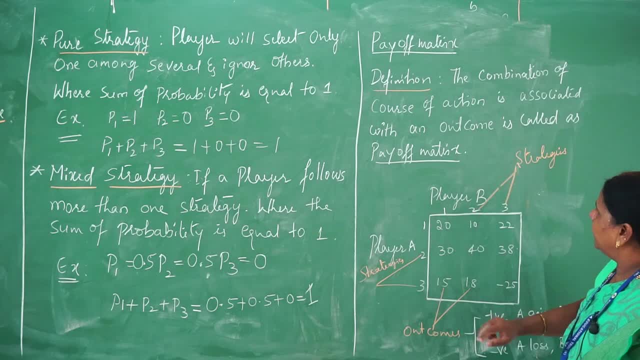 two players are identified: player A and player B. They are identified by the three strategies of A and B, respectively 1, 2, 3 for the player B, 1, 2, 3 for the player A, and wherever the each player strategy of an A and B is intersecting. 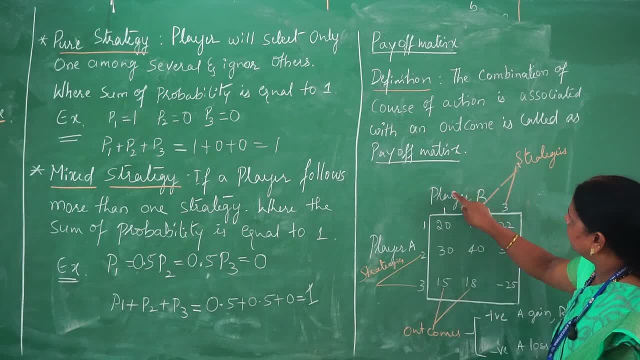 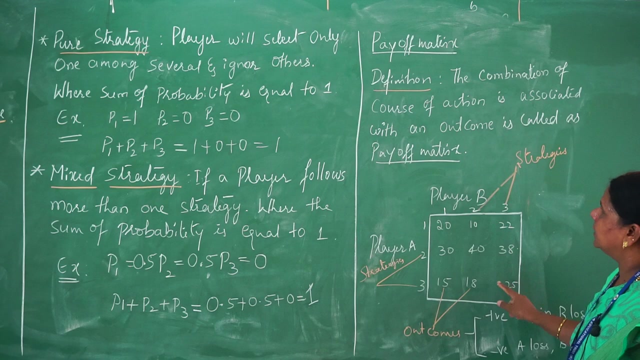 For example, player A1 is intersecting with the player B, then this is called as an outcome. These entries of the matrix will be identified as an outcomes of the matrix and this matrix is called as an payoff matrix And all these outcomes are considered as an course of action. that is nothing but strategies. 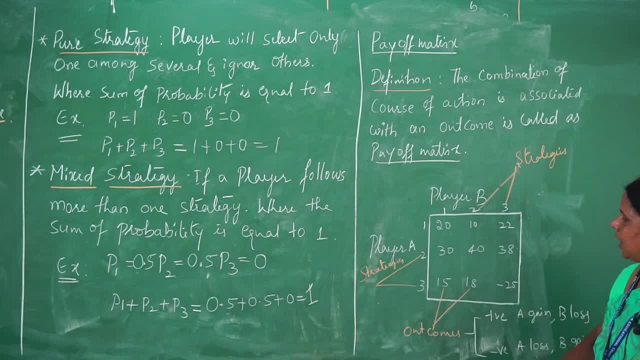 The course of action, whichever we are defining in terms of an outcome, will be defined in terms of an two types of an different value. One is called as an positive, Another one is called as a negative. If the outcome is positive, then player A will get a gain and player B will get a loss. 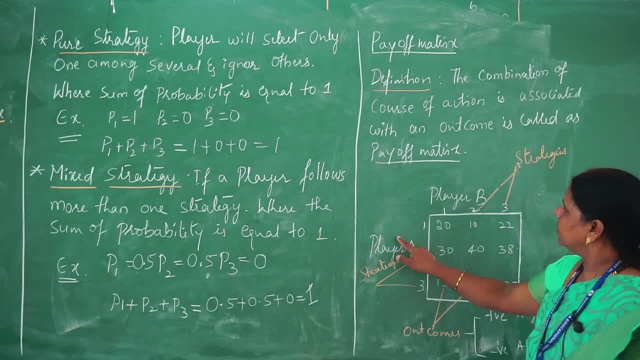 If the outcome is negative, A is going to get a loss but player B is going to get a gain. So these will be evaluated with the one of the example. Let us we will see how that entire loss and gain is going. 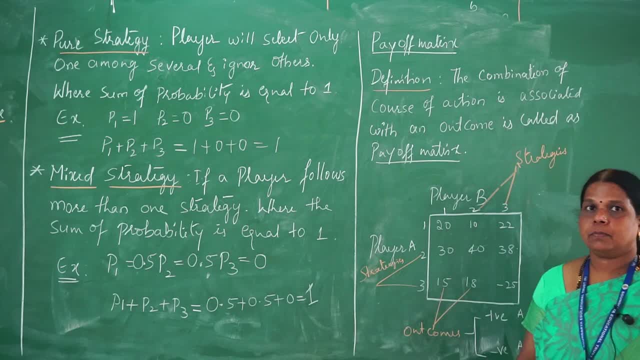 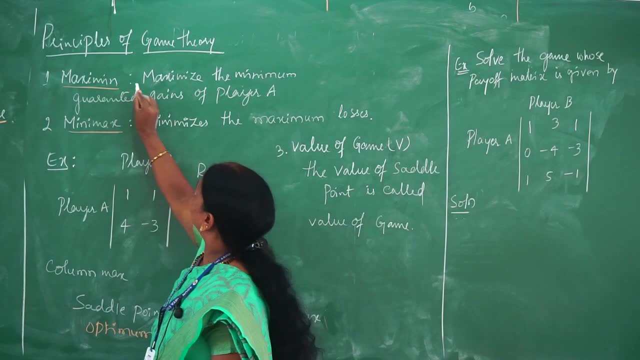 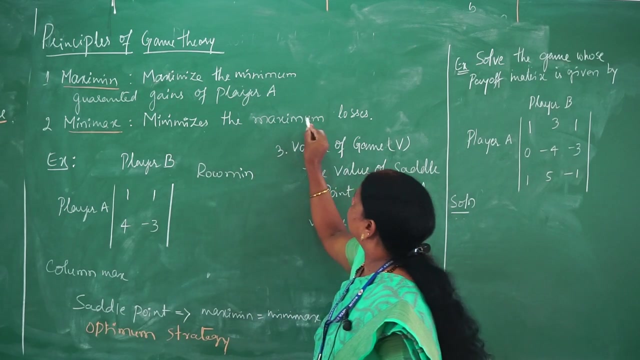 to be evaluated with the one of the example Principles of gain theory: maximin and minimax. In the maximin maximize the minimum guaranteed gain of player A. In minimax minimizes the maximum losses. So that we will discuss with the example- small example- Along with these. 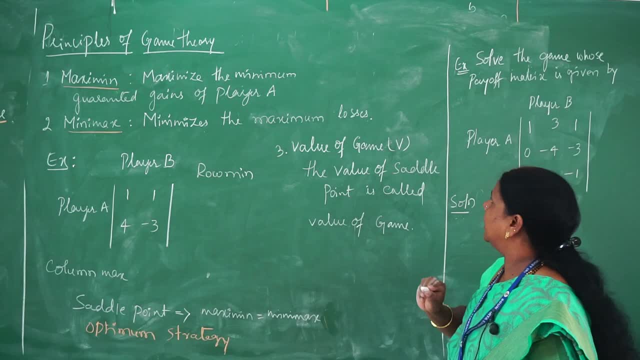 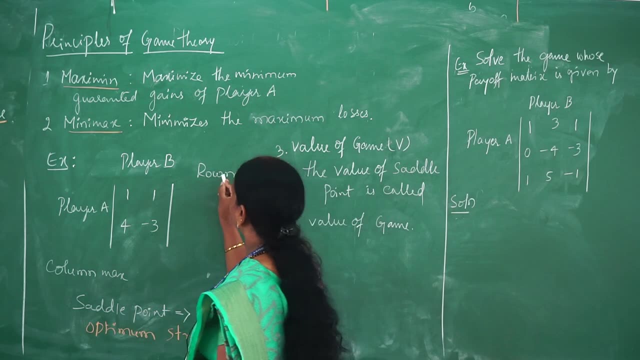 maximin and minimax. we need to find out the value of a game, The value of the game. if you wanted to find out first, you need to find out the saddle point. The saddle point is nothing, but where row maximin and minimax will intersect, that point. 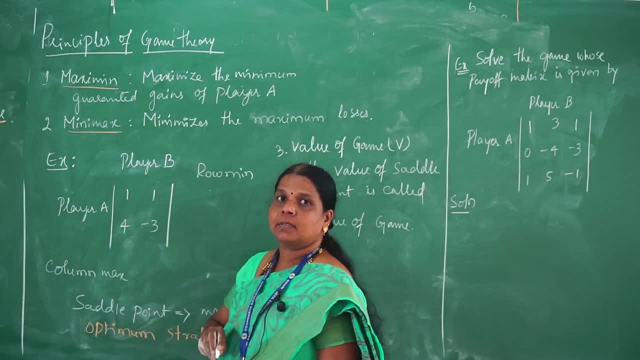 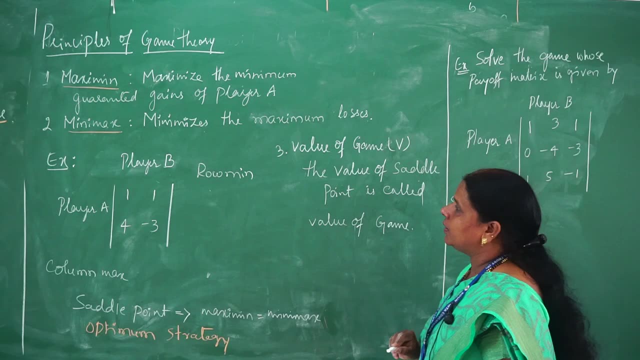 What is called as an saddle point. The value of the saddle point itself is called as an game value. So how to evaluate this game value As well as the saddle point, we will check with the two principles of the game theory called as a maximin and minimax values. 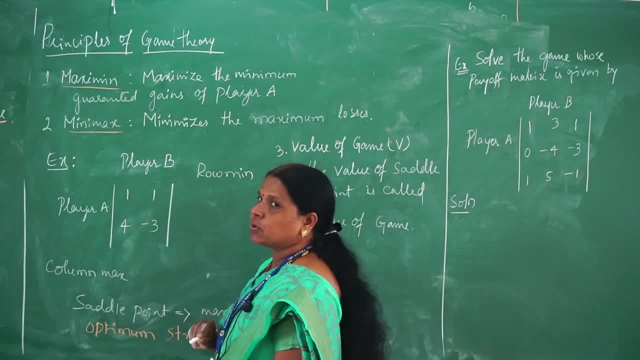 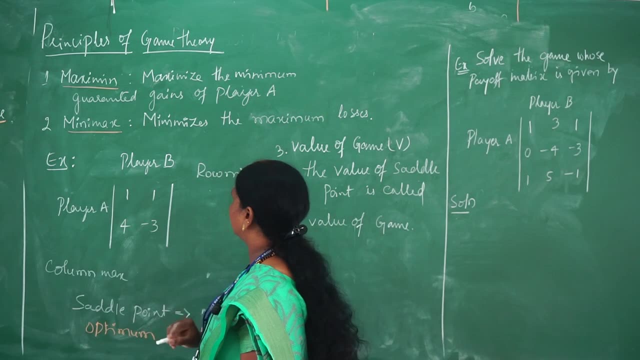 So here I took a one example. So with the 2 cross, 2 matrix, square matrix, player A, player B, with the values 1, 1,, 4, minus 3.. So in this example we need to find out the. 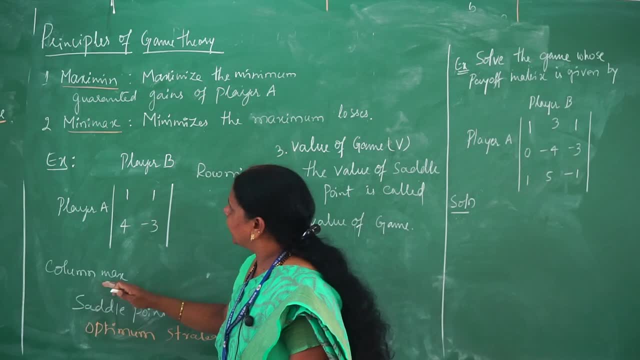 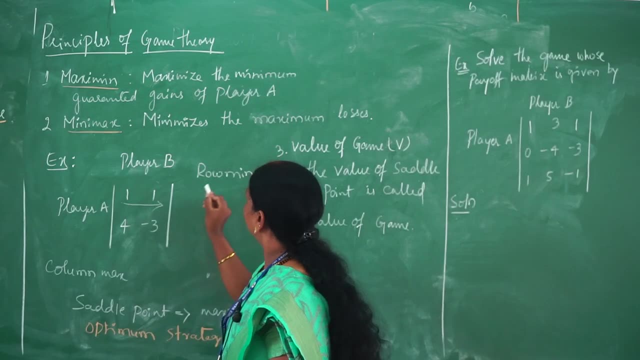 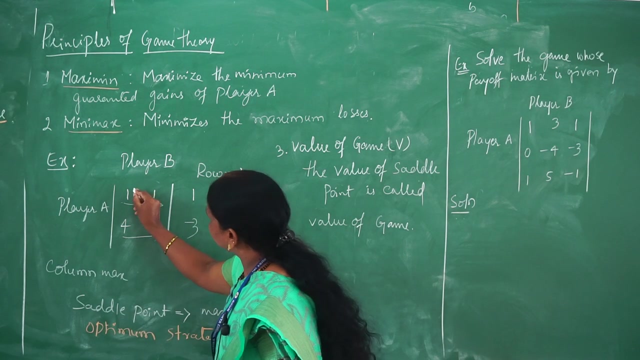 row minimum for the row value and column maximum for the. each column existed in the matrix In this row. if I consider a row 1, in this row the minimum value is 1.. In this second row the minimum value is minus 3.. I will consider a column now because I need to find. 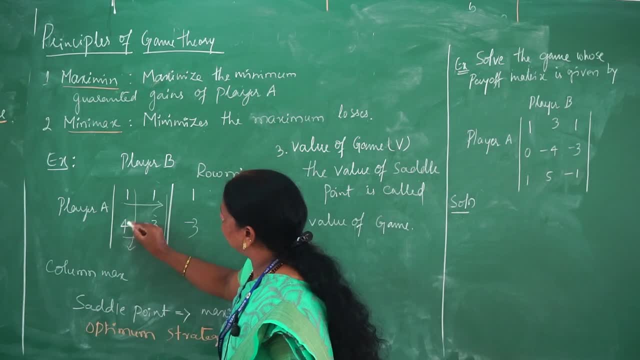 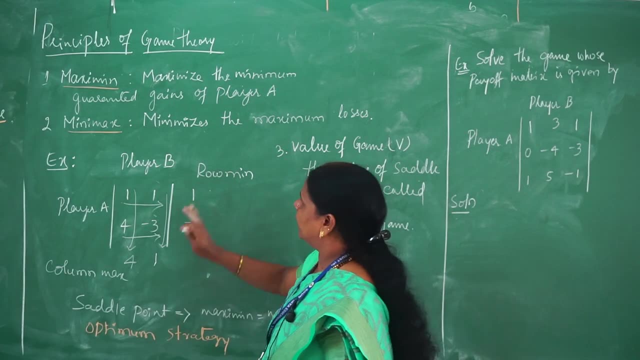 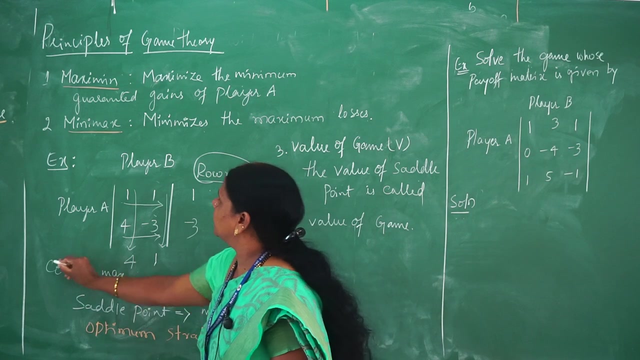 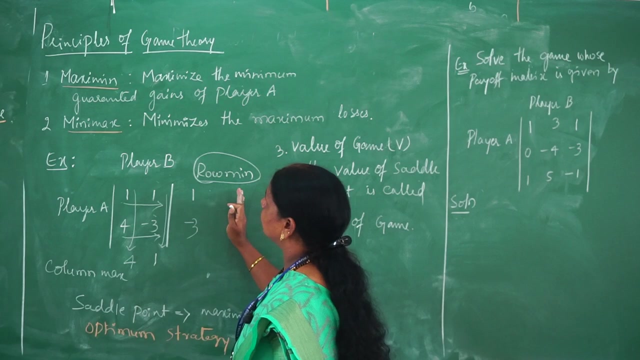 out maximum value of the column. in this column the maximum value is 4 and in this column the maximum value is 1.. evaluated two different values of the game game theory. called as an row minimum as well as maximum column maximum, and it will be called as an. called as an finding the minimax as. 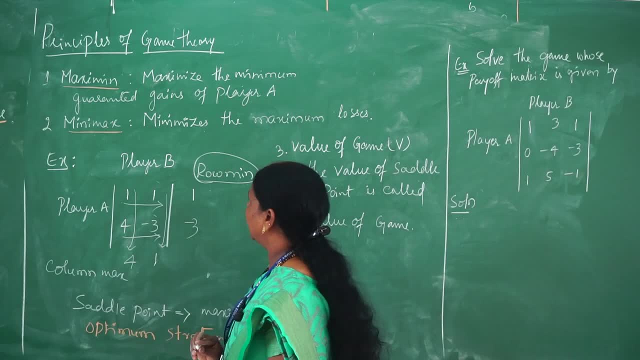 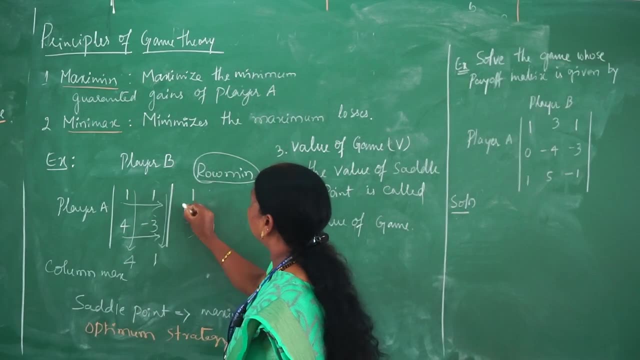 well as max mini properties of the game theory. So as soon as we evaluated row min value, you need to find out which one is the minimax minimum max value. that has to be evaluated first. So from these two value, this is the minimum max value and from these two value we need 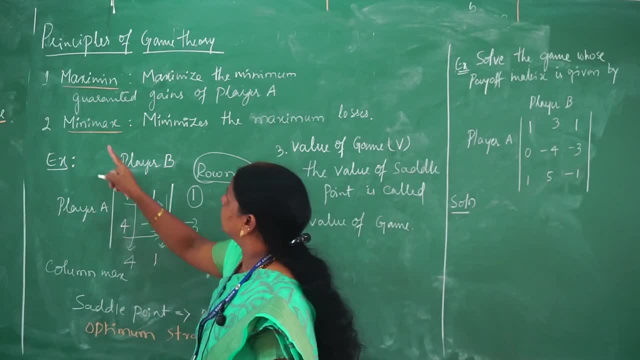 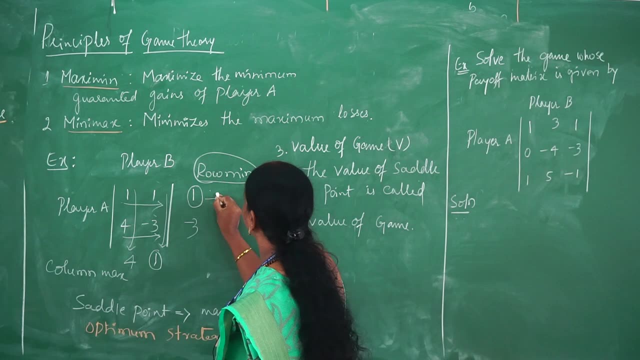 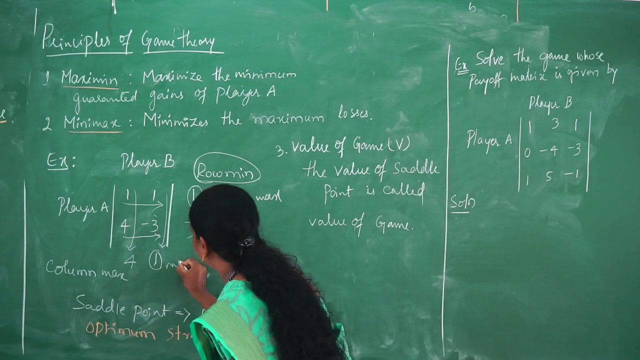 to find out maximum min value. that is called as an maximin. among these two maximum value, the minimum value is this one. So now this value is called as an minimax and this is called maximini. where these two points are intersecting, that cell value itself is called as an saddle point. 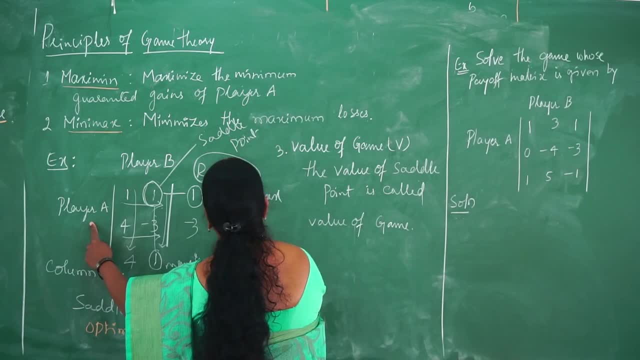 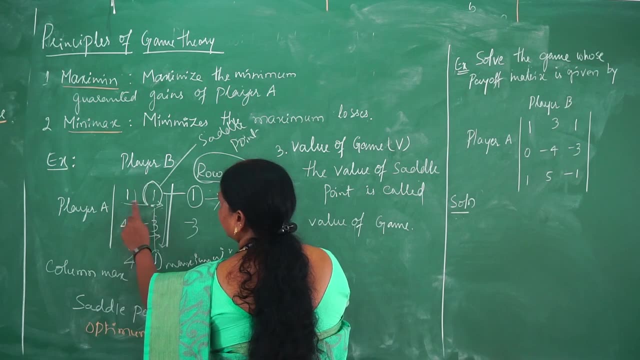 So now saddle point will be defined like this: SP equals to player A, the row is second row, first row, sorry, first row, second column. So I will define this as an A1- B2. so the position of saddle point is A1- B2.. The value in this column is A1- B2.. 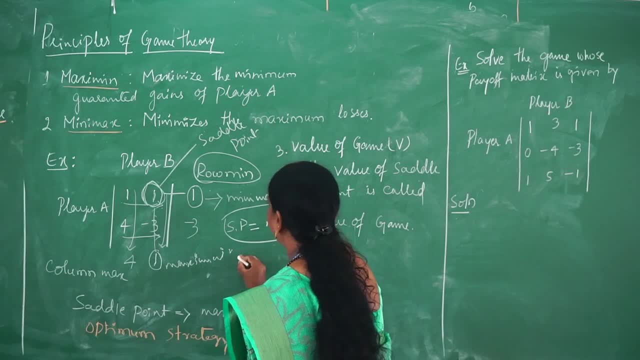 So I will define this as an A1- B2.. So the position of saddle point is that cell is called as an 1.. The game value of this one will be denoted by V. V equals to the value is 1.. So where both the saddle points, where both maxmin and minimax is intersecting that value. 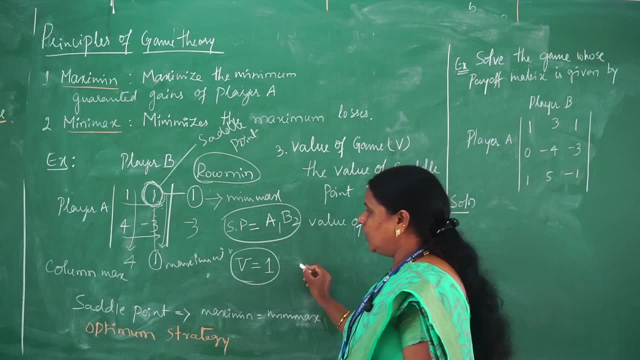 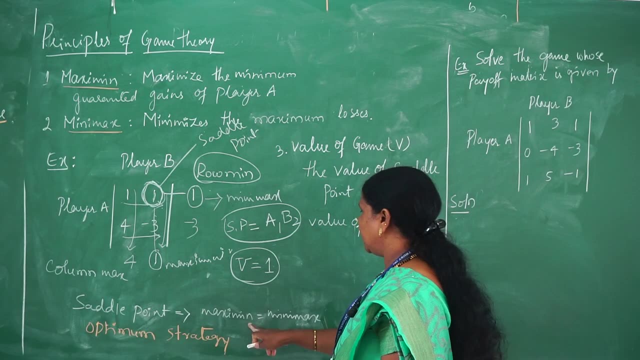 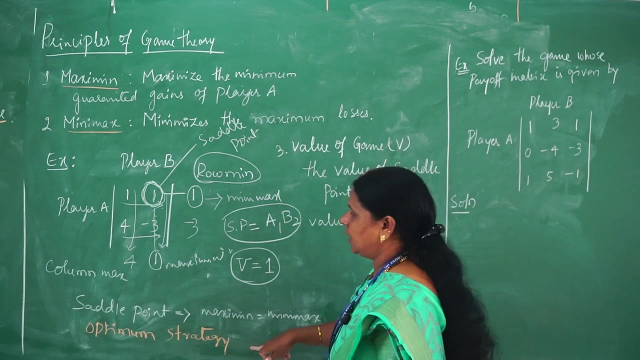 is itself called as an game value. So now here we how we should find out. the saddle point is identified where both maxmin and minimax value are equal to each other, then that game is called as an optimum strategy game. or we can say this game: pay off game. 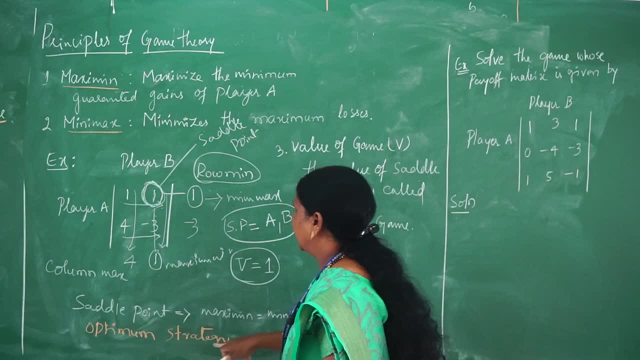 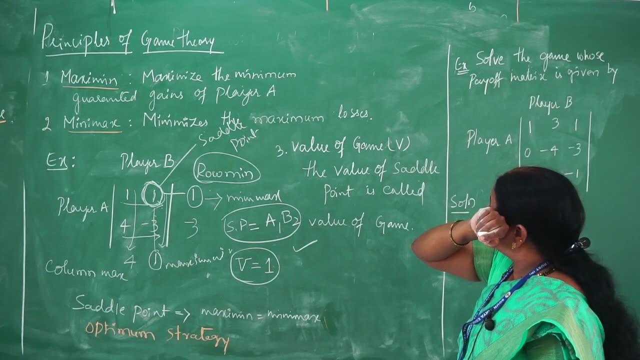 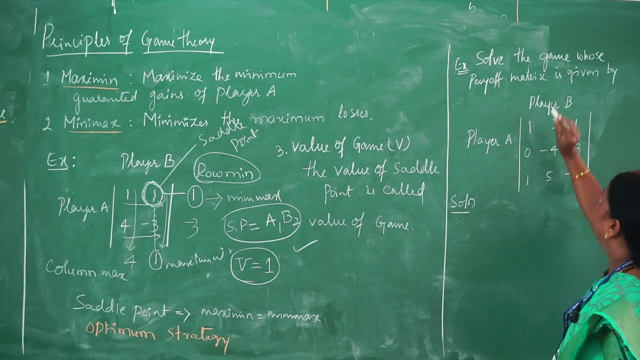 matrix will be evaluated by optimum strategy game. So this is the one type of an principle: how we are going to be evaluated with the two properties. one is called as a maximin, another one is minimax. Moving to the one of the example, solve the game whose pay off matrix is given by, like 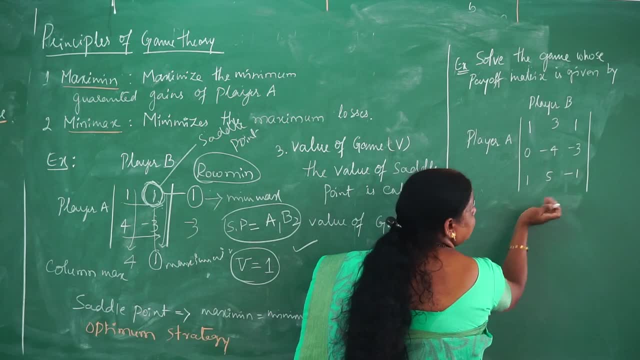 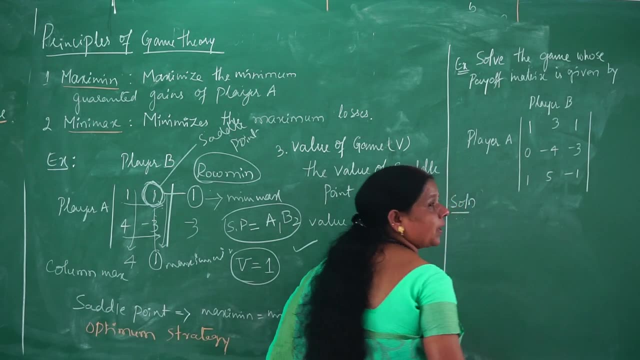 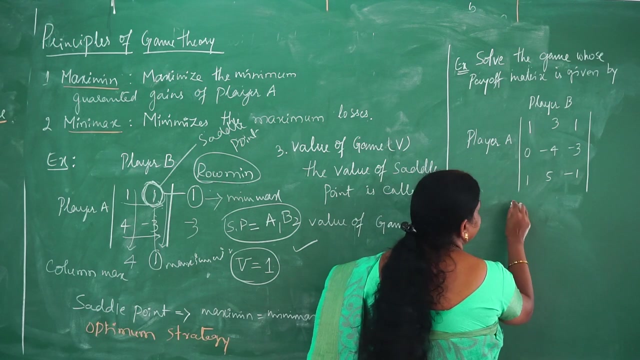 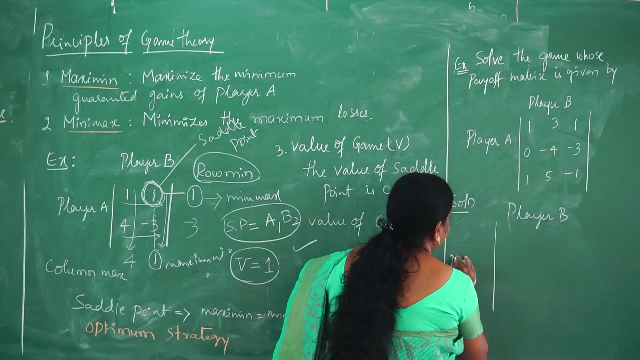 this, player A, player B, with a 3 cross 3 matrix. now we need to find out maxmin as well as minimax value for this matrix, to identify what is the saddle point, along with the game value. So now, first you find out as it is, you write down the matrix. player B, player A, values are: 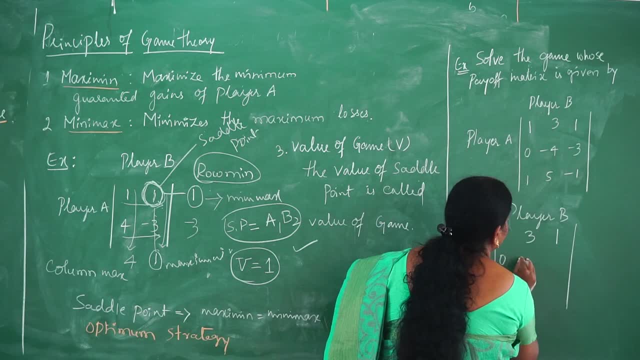 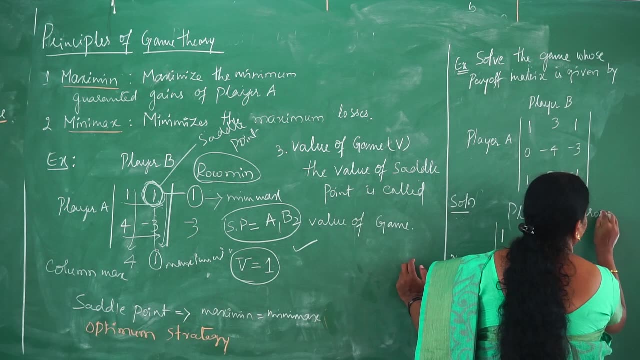 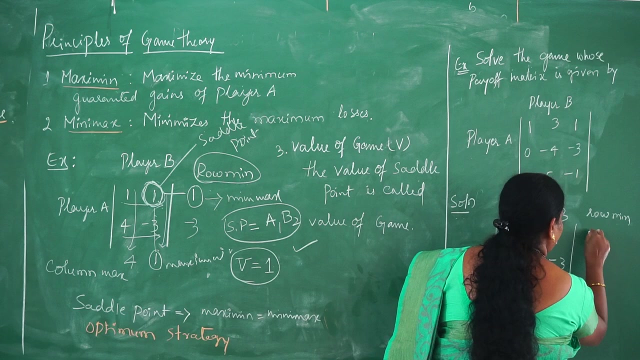 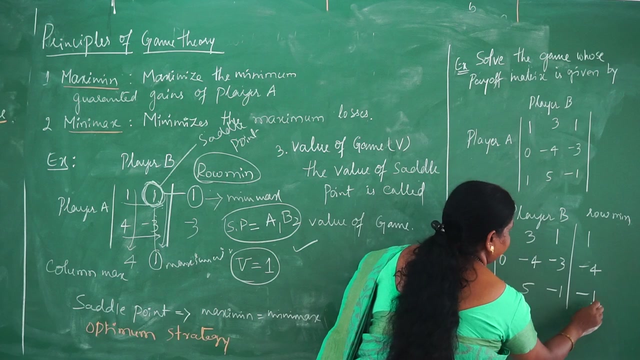 like this: 1, 3.. 1, 0 minus 4 minus 3. 1, 5 minus 1. here we need to find out row minimum value and here we need to find out column maximum value. So row minimum for this one is 1, for this is minus 4, for this is minus 1.. 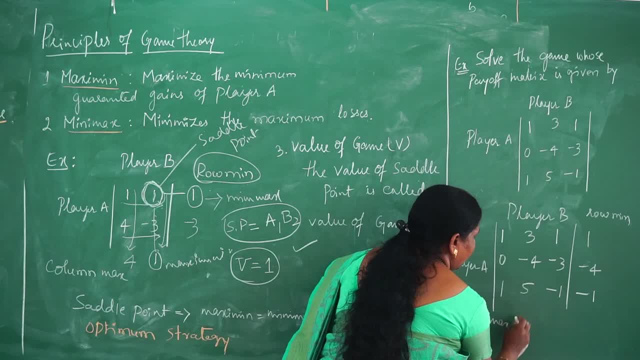 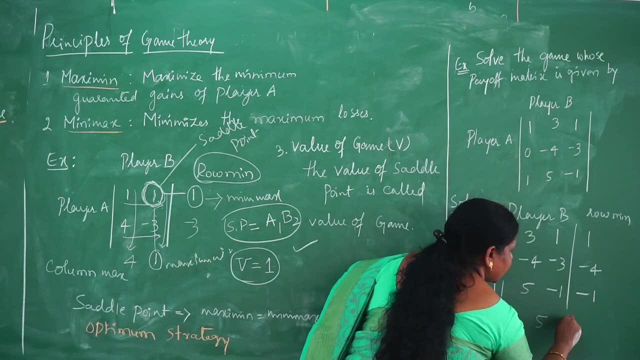 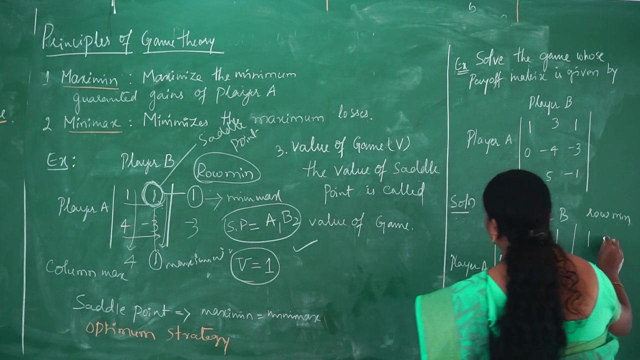 For column, we should find out maximum value. here. the maximum value for the first column is 1. for the second column, value is 5. for the third column, the value is again 1.. So now, after finding row minimum and column maximum, we need to find out minimax value. 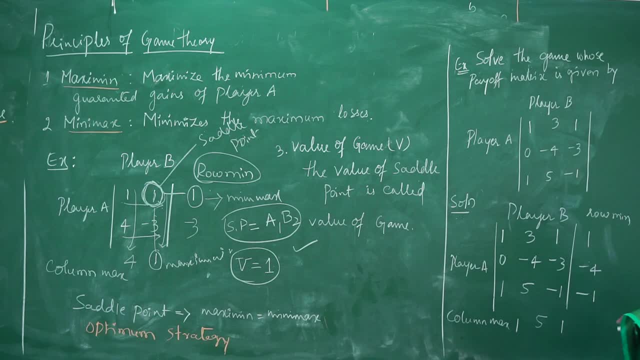 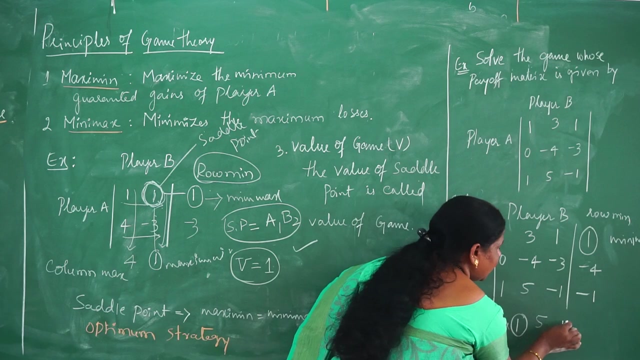 for row min. So now, among these two, which one is the maximum? this one is the maximum, So it will called as an minimax. So among these maximum value, we need to find out minimum value. Here there are two minimum value. 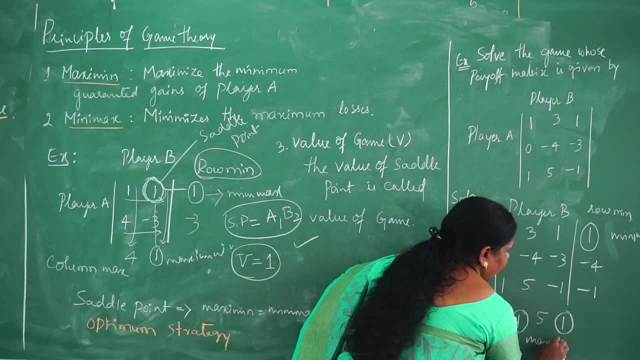 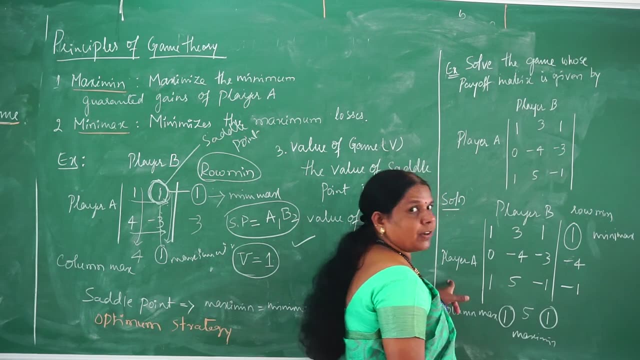 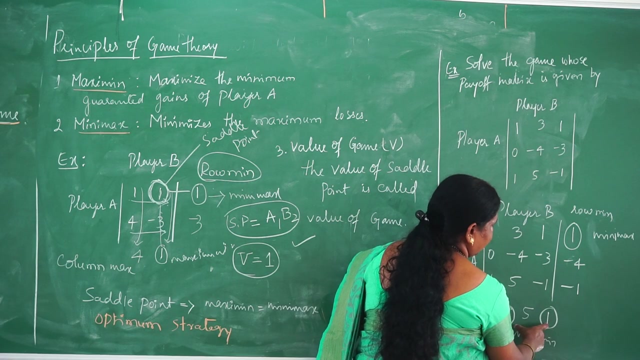 So these will be called as an maximin values. So now how we should find out the strategy for this pair of matrix. There are two different types of an strategy for this. one, Because in the column maximum we got two minimum value with the two different position. one 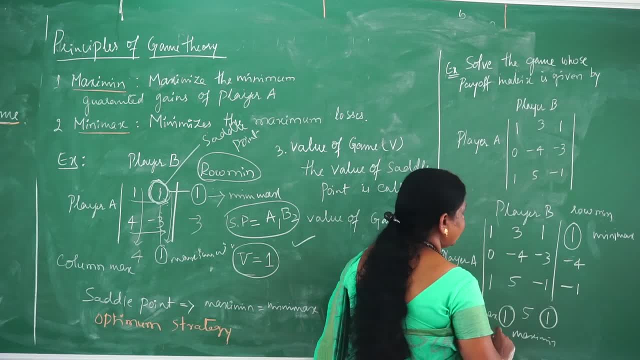 is at the A1.. Another one is at the A3. So in the column maximum we got two minimum value with the two different position. So that is why what we need to do First, we need to intersect these two points. which one is there? 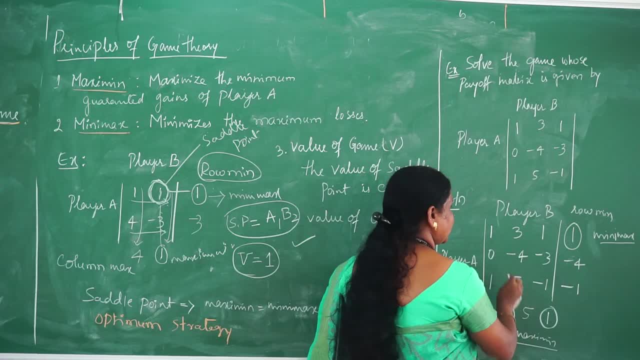 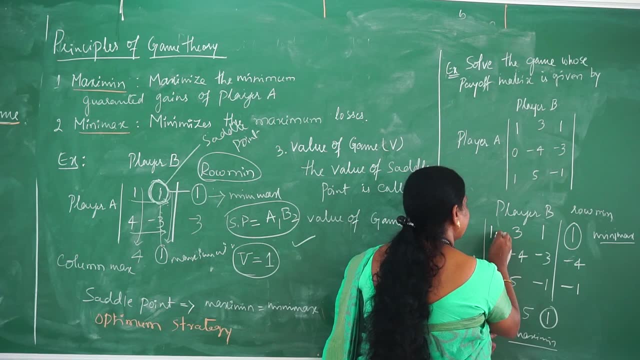 in the mini max position as well as in the max mini position to find out the saddle point. If I consider this one, so it has to intersect like this. So now this is called as an saddle point. that is nothing but sp. So saddle point is intersecting at the position a1. b1 is the first. 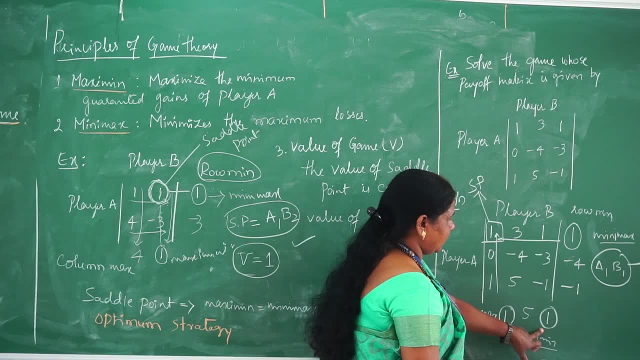 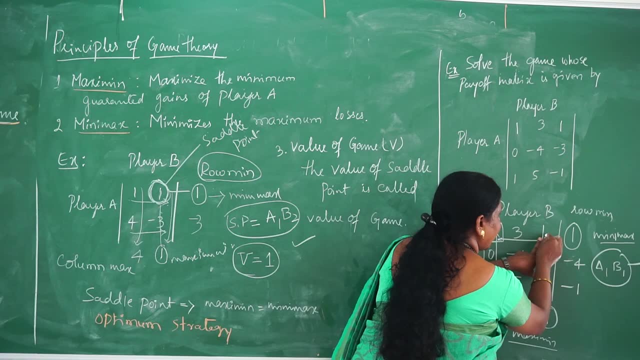 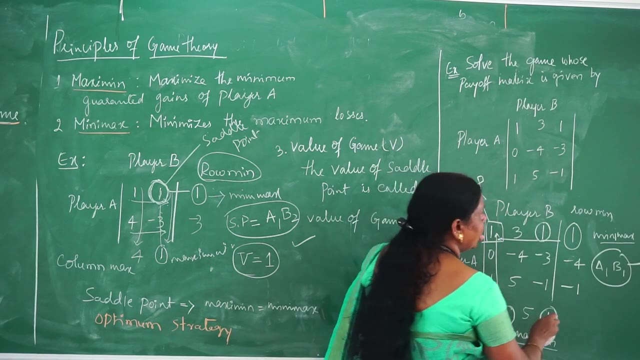 strategy. So next one again here. one is there same. So one is intersecting with the another mini max value in the third column, with the first row. So now this is also considered as saddle point for the game of. So now it can be read as a1- b3. this is called a second strategy. 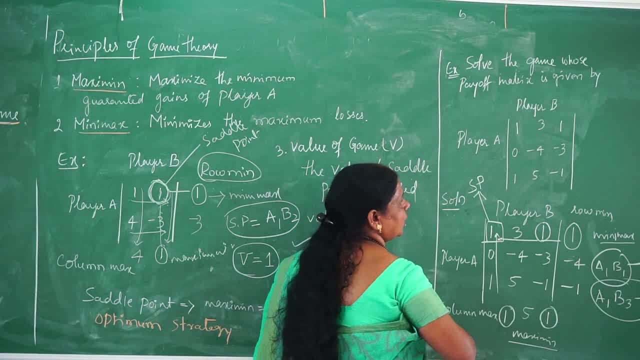 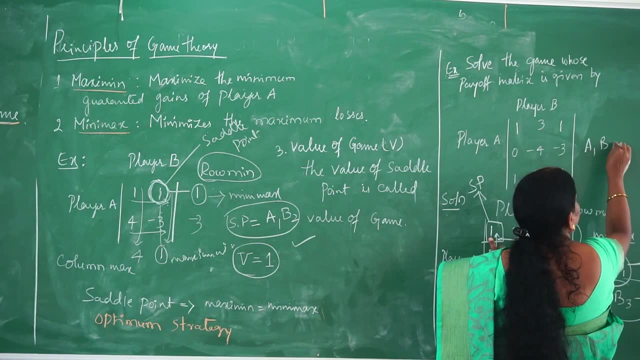 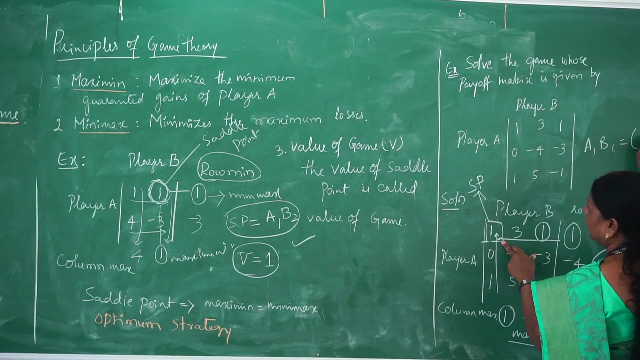 for the payoff matrix. Among these, choose any one for finding. So now I will consider a1- b1.. So when I consider a1- b1, I need to find out here probability. that probability is always equals to 1, because that we studied in the beginning. So each